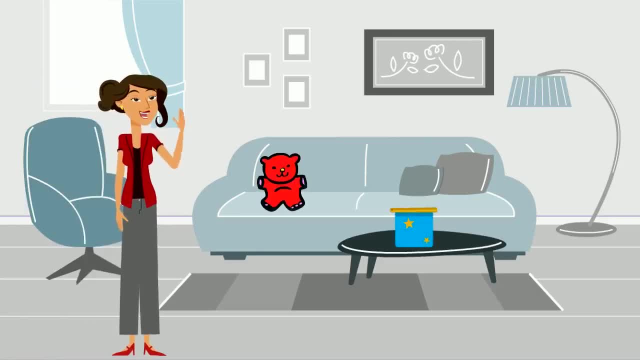 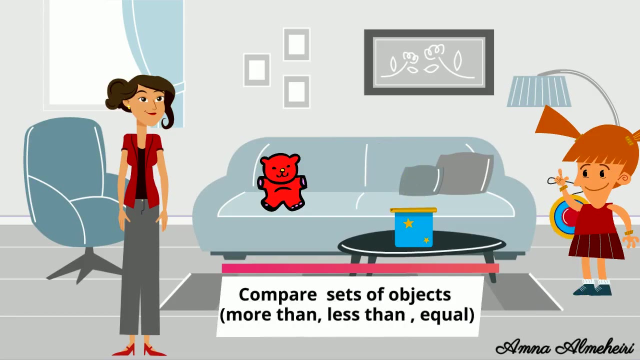 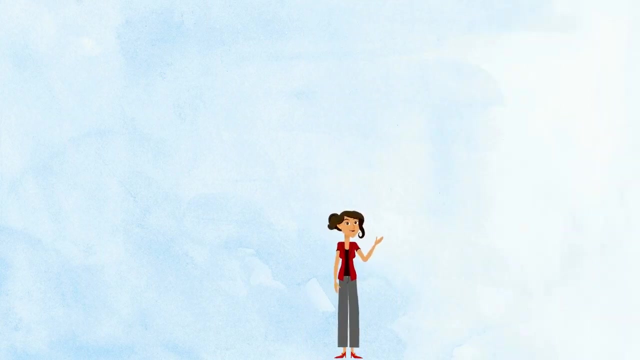 Hello kids, how are you today? I hope that you are feeling good. Today is Wednesday and we have math. I hope that you are ready for a new math lesson. It's very easy. We are going to learn about comparing sets of objects, But before we start, I need to make sure that you are following the rules. Do you remember what they are? Very good Eyes looking. 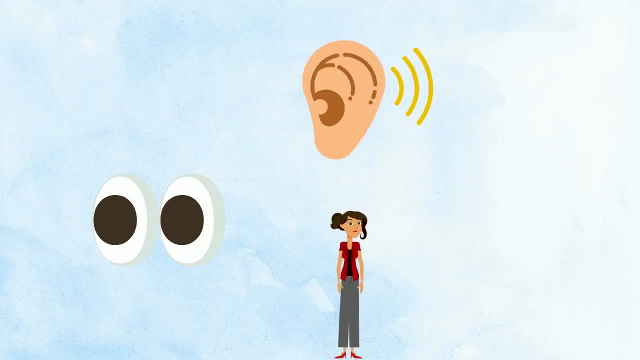 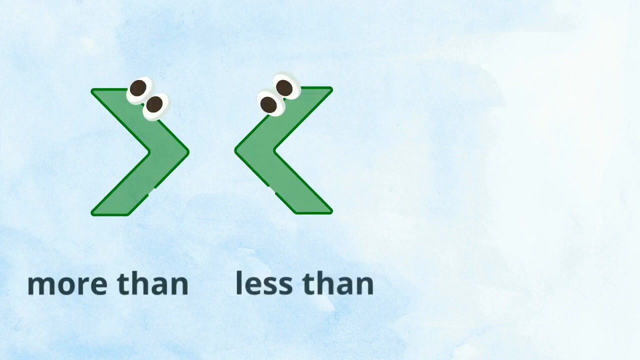 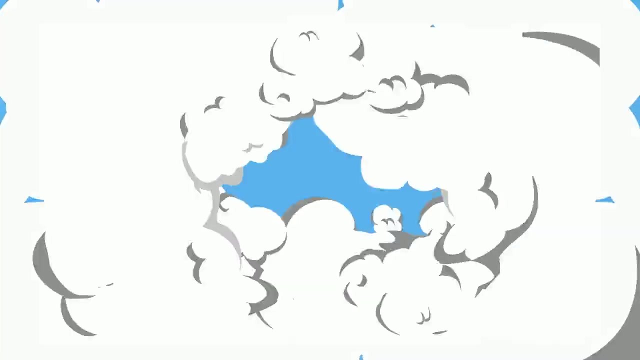 Ears listening And mind awake. Let's start learning about three symbols in math. The first one is more than, The second one go less than And the third one refer to equal. When you use the symbol kits, just think of it as it is. 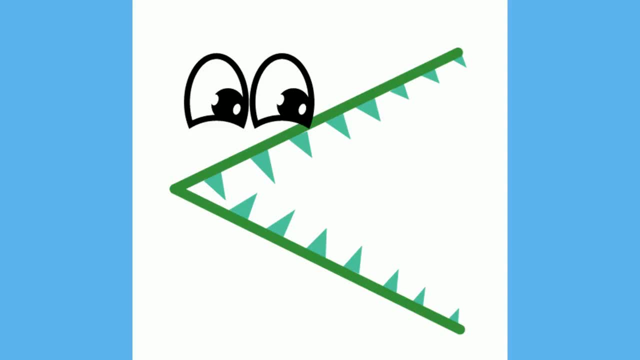 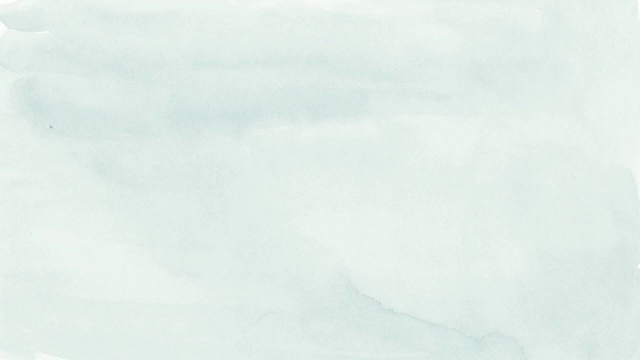 A big mouth, A big mouth of a crocodile who is feeling always hungry and need to eat the biggest number. So the open side will always face the biggest number. But the question here: for what do I use the symbols? Look at the picture. How many apples do I have? I have five apples, Good job. 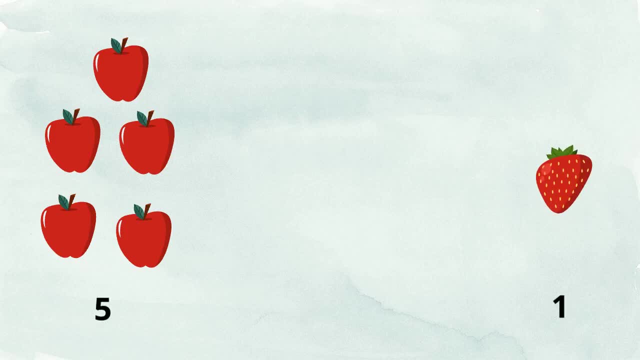 And how many strawberries I have one strawberry. Now look at the groups. Which group has more, The apples or the strawberry? Well done, The apples is more than the strawberry. So the big mouth of the crocodile will face the apples. It's more than the strawberry. 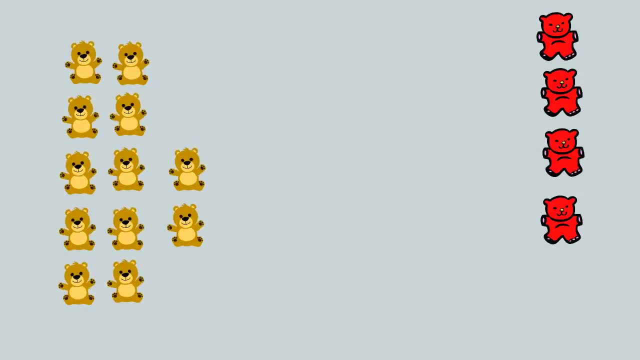 Let's look here: How many brown teddy bears, How many brown teddy bears, How many brown teddy bears do we have? Let's group it to tens and ones. We have one group of ten and two ones. That makes twelve. 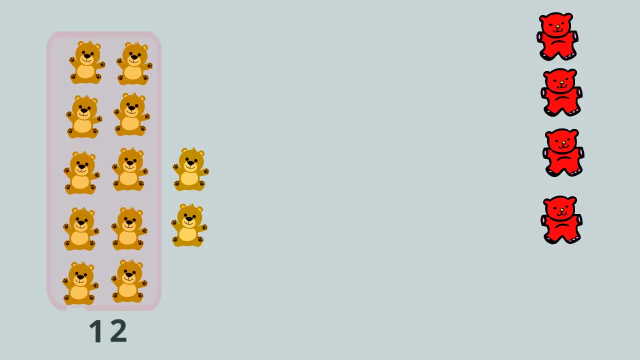 And how many red teddy bears do we have? We have four red teddy bears. Now look at the sets. Which one has more? The brown teddy bears or the red teddy bears? Well done, The brown teddy bears has more.